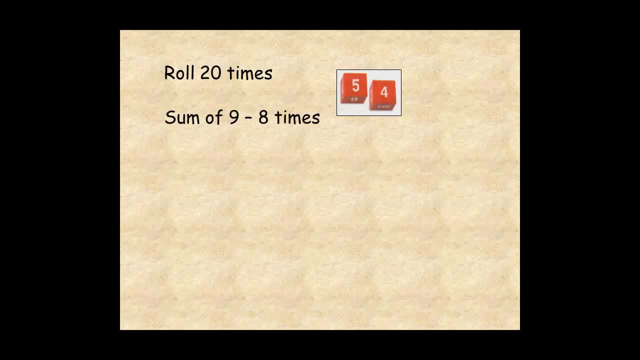 and the sum of nine comes up eight times. Now the theoretical probability is four chances out of 36, because there are four combinations that add to nine And when rolling two dice there are 36 possible outcomes. Then 4 over 36 simplifies to 1 over 9.. 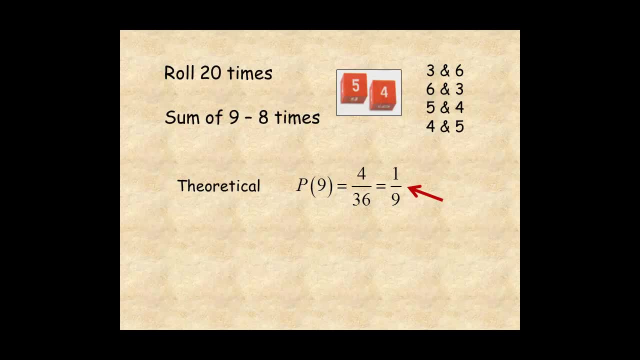 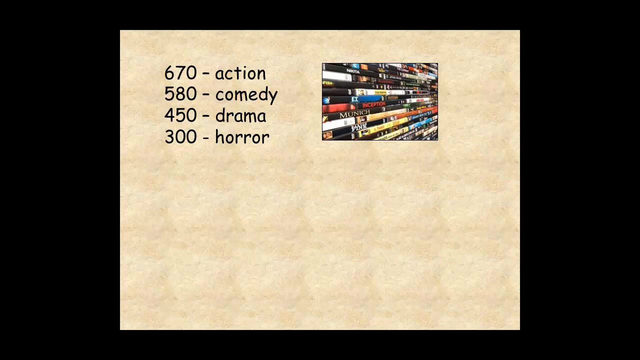 The experimental probability is 8 over 20, which simplifies to 2 over 5.. In this case, the theoretical and experimental probabilities are not close. One possible explanation is that there were not enough trials. Theoretical and experimental probability can be used to make predictions of future events. 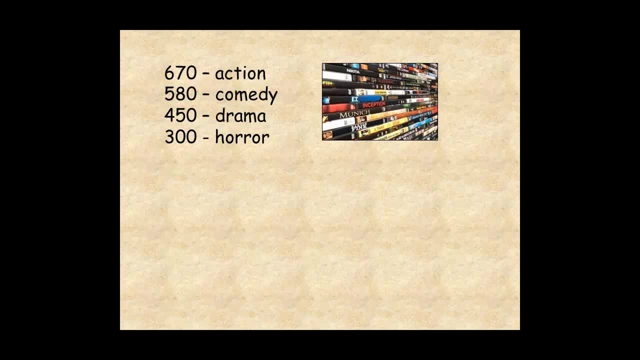 For example, here's a list of DVDs sold last year by a certain store. Out of 2,000 DVDs sold, 580 were comedies. So the probability that a customer will buy a comedy DVD is 580 over 2,000,. 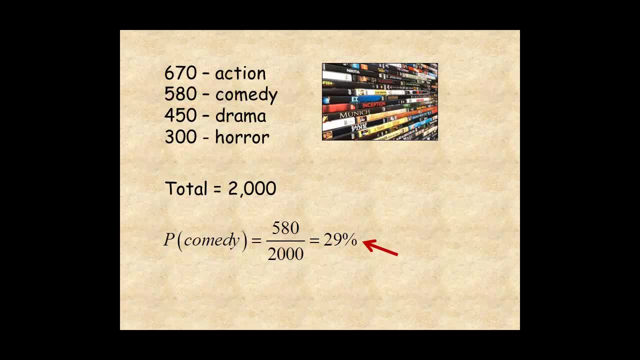 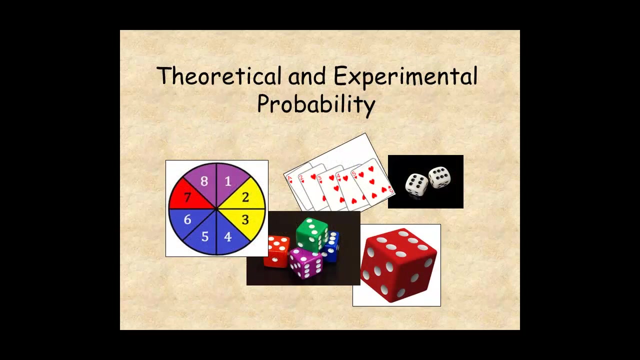 or about 29%. Then, assuming this trend continues, when buying 5,000 DVDs for this year, the owner should make 29% of them comedies. This lesson helped you understand the difference between theoretical and experimental probability, And this lesson was brought to you by the MathFun Academy. 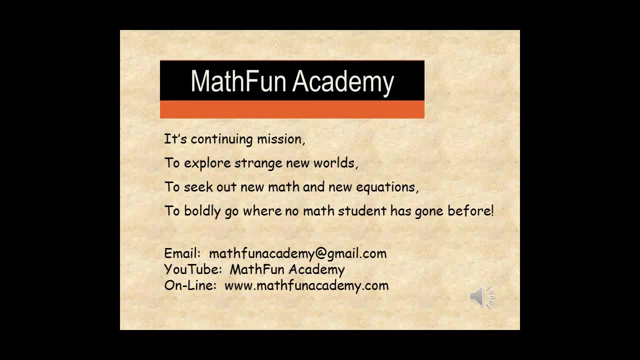 its continuing mission to explore strange new worlds, to seek out new math and new equations, to boldly go where no math student has gone before: wwwmathfuncom, wwwmathfuncom, wwwmathfuncom.